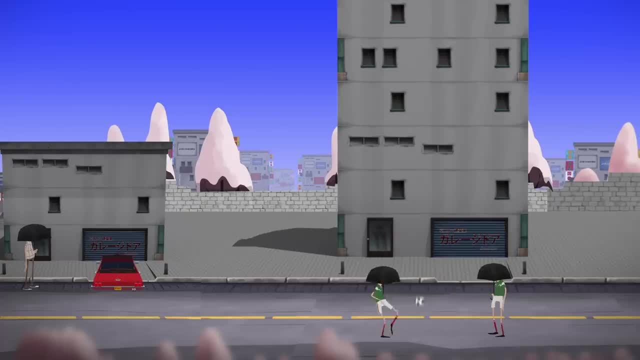 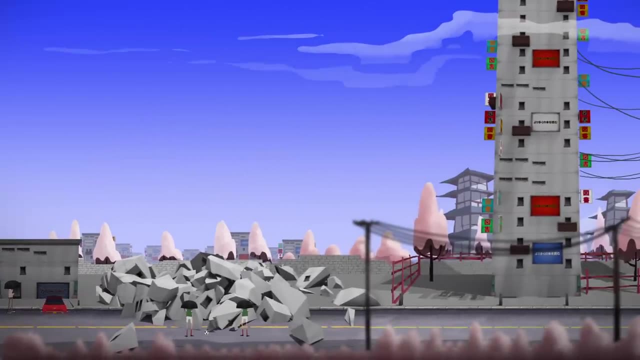 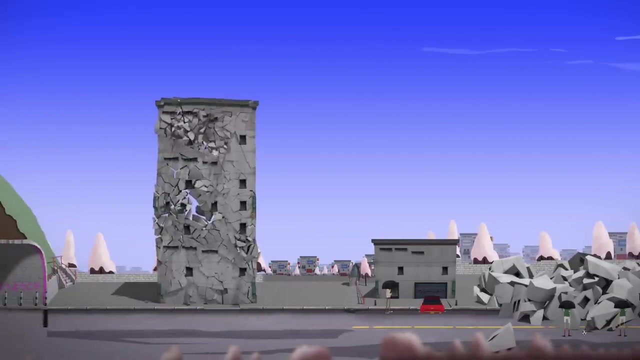 many buildings between 6 and 15 stories tall collapsed. What's strange is that, while shorter buildings nearby did keep standing, buildings taller than 15 stories were also less damaged, and the mid-sized buildings that collapsed were observed shaking far more violently than the earthquake itself. 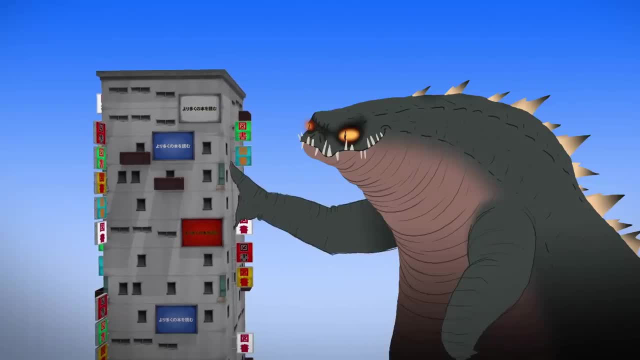 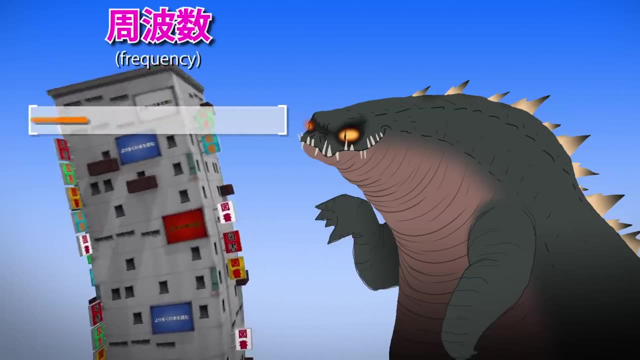 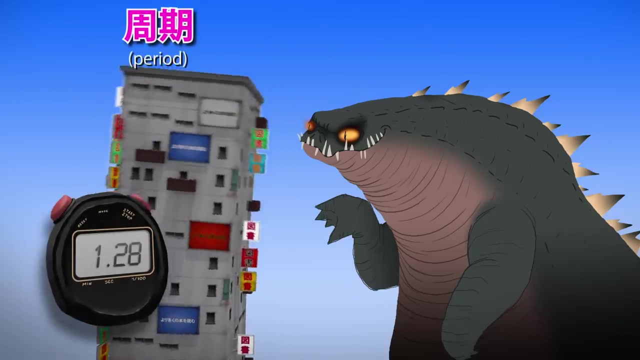 How is that possible? The answer has to do with something known as natural frequency. In an oscillating system, the frequency is how many back and forth movement cycles occur within a second. This is the inverse of the period, which is how many seconds it takes to complete one cycle. 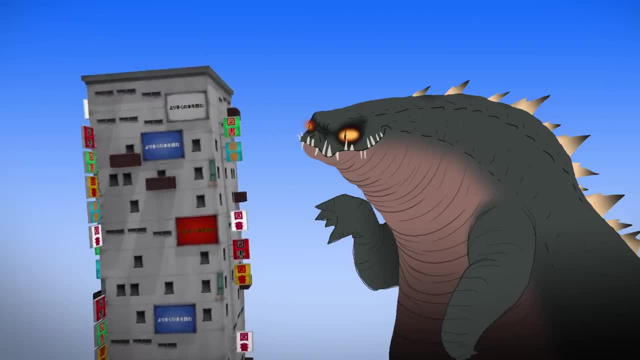 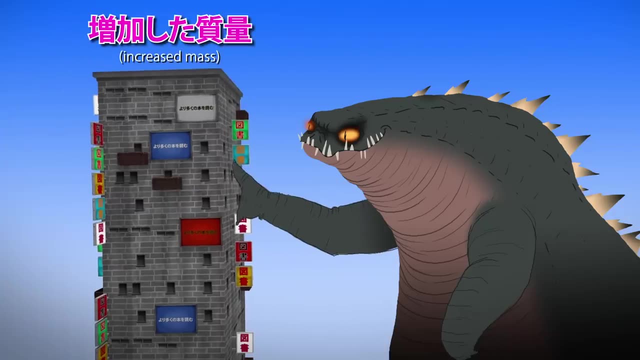 In a building's natural frequency, determined by its mass and stiffness, is the frequency that its vibrations will tend to cluster around. Increasing a building's mass slows down the rate at which it naturally vibrates, while increasing stiffness makes it vibrate faster. 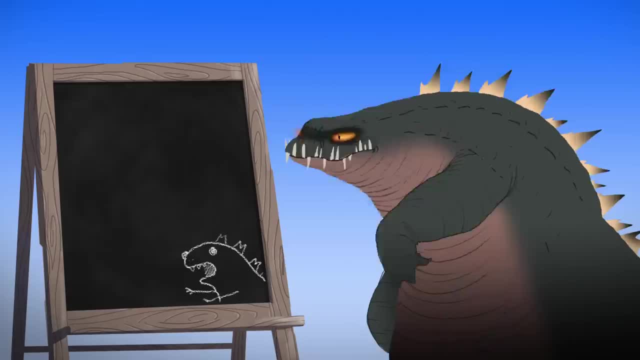 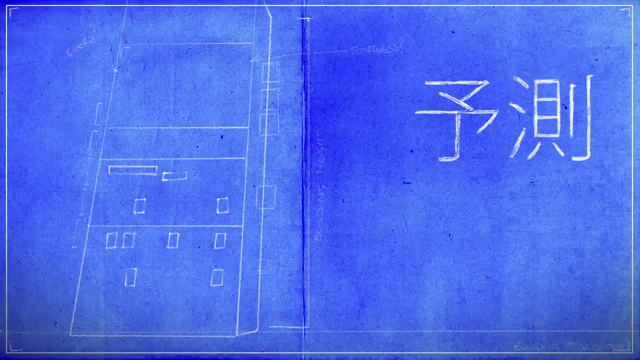 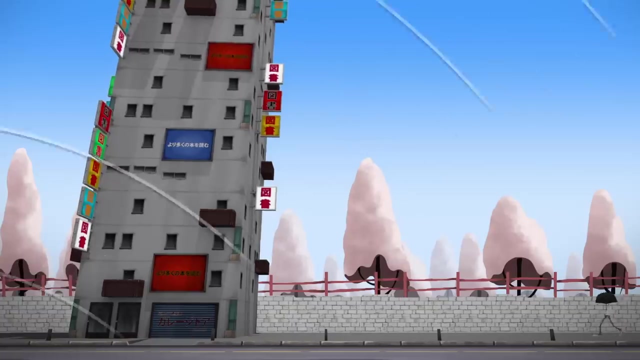 So in the equation representing their relationship, stiffness and natural frequency are proportional to one another, while mass and natural frequency are inversely proportional. What happened in Mexico City was an effect called resonance, where the frequency of the earthquake's seismic waves happened to match the natural frequency of the mid-sized buildings. 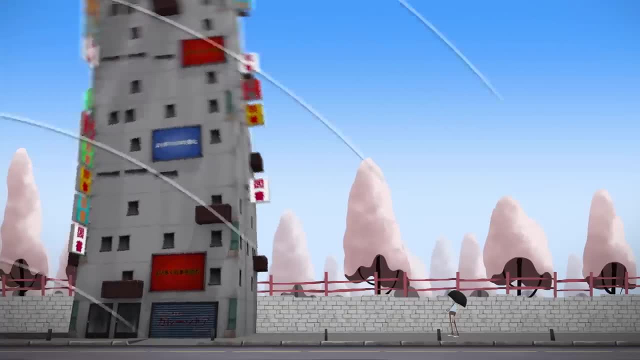 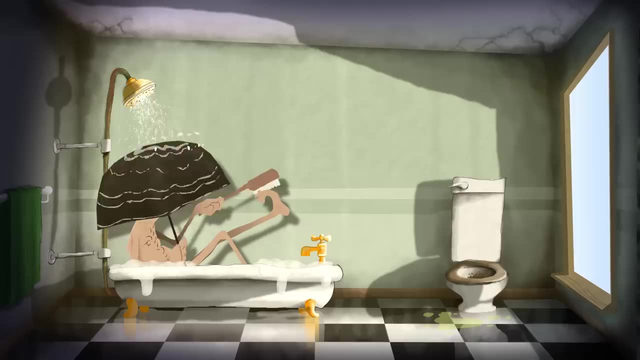 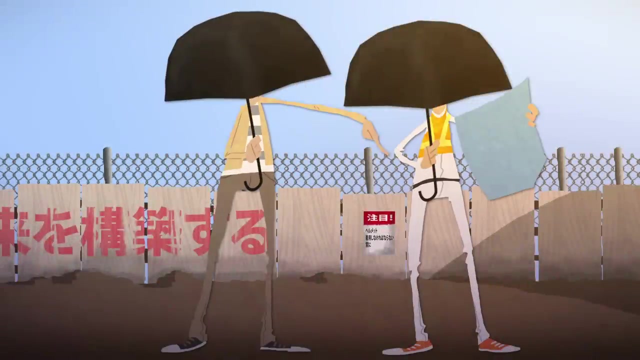 Like a well-timed push-on-a-swing set. each additional seismic wave amplified the building's vibration in its current direction, causing it to swing even further back and so on, eventually reaching a far greater extent than the initial displacement. Today, engineers work with geologists and seismologists. 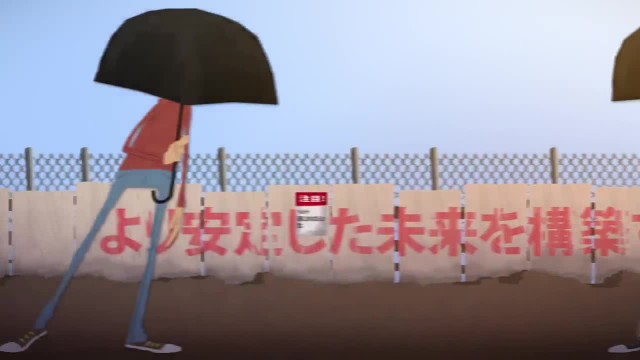 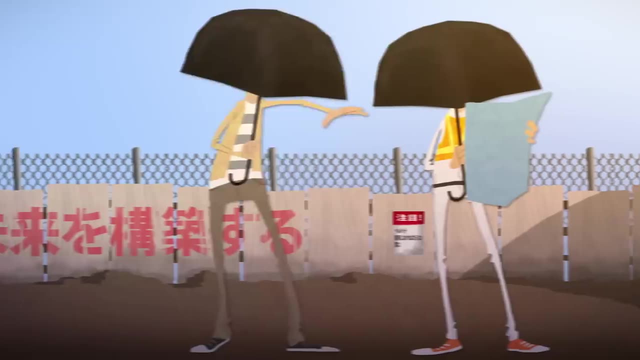 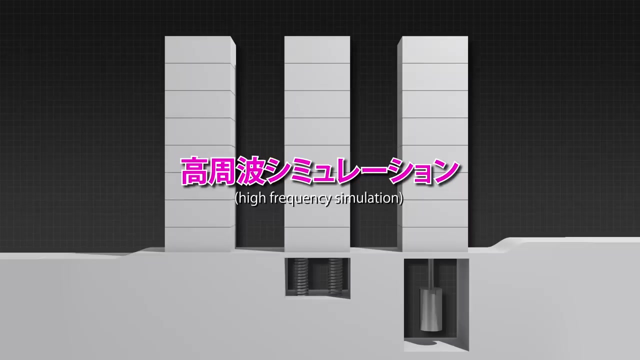 to predict the frequency of earthquake motions at building sites in order to prevent resonance-induced collapses, taking into account factors such as soil type and fault type, as well as data from previous quakes. Low frequencies of motion will cause more damage to taller and more flexible buildings. 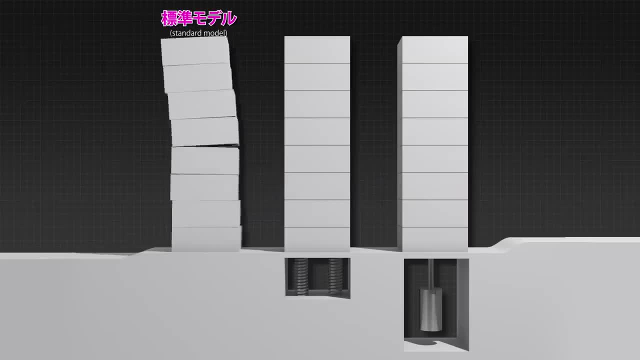 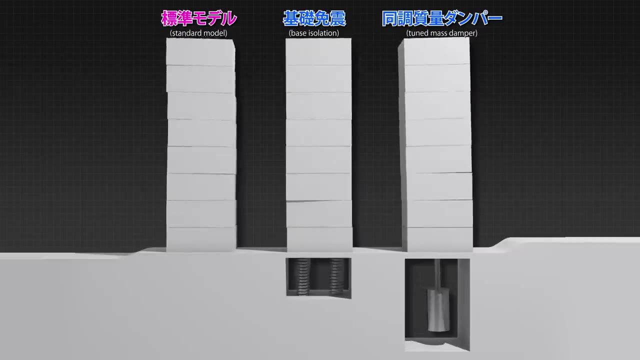 while high frequencies of motion pose more threat to structures that are shorter and stiffer, Engineers have also devised ways to absorb shocks and limit deformation using innovative systems. Base isolation uses flexible layers to isolate the foundation's displacement from the rest of the building, while tuned mass damper systems cancel out resonance. by oscillating out of phase with the natural frequency to reduce vibrations. In the end, it's not the sturdiest buildings that will remain standing, but the smartest ones.